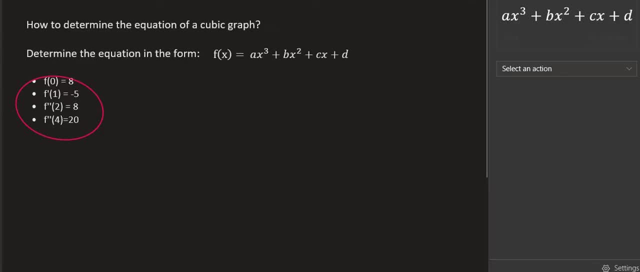 information that they've given you and you plug it into the appropriate equation one by one. So let's start with the first one. They're telling us that they want you to plug it into the graph of f, which is this one. They're saying that when x is zero, the answer should be eight. So we can. 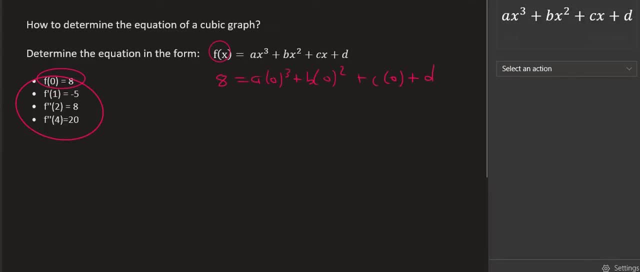 do this, Okay. so you see what I've done there. I've literally plugged in all the x's as zero and I've made the answer equal to eight, because that part cancels and that part cancels, And so that allows us to find that d is eight. You see, so we've already found one letter. now. Now the 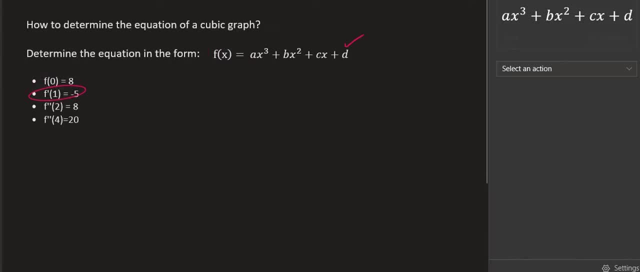 next one says that we should plug the x value of one into the correct equation. So we're going to plug the x value of one into the correct equation. So we're going to plug the x value of one into the first derivative. So let's go get the first derivative. That's going to give us three: a, x. 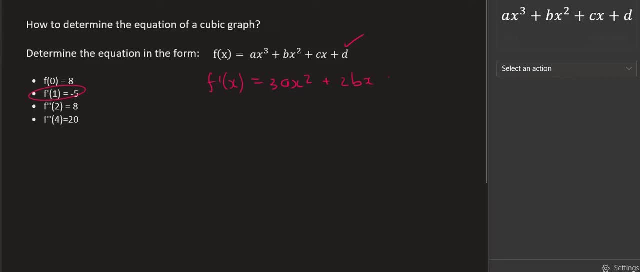 squared plus two, b, x plus c, and then the d would fall away. They tell us that the answer is minus five when x is one. So you see, guys, what I'm doing. I'm literally just plugging in. I'm not even thinking about this one, I'm just plugging things in, And then you simplify as far as 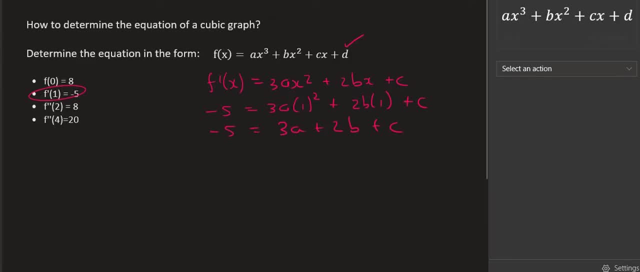 possible And unfortunately there's no other. on what? we can't get any answers from that. So we're going to plug an x value of two into the second derivative. So the second derivative is going to look. let's just write down the first derivative again. So that's three, a x squared plus. 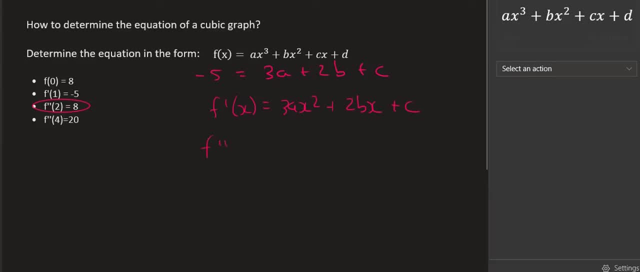 two b x plus c, Then the second derivative will be six a x plus two b. They tell us that when x is two, then the answer should be eight. That and then eight is equal to 12 a plus two b. We could. 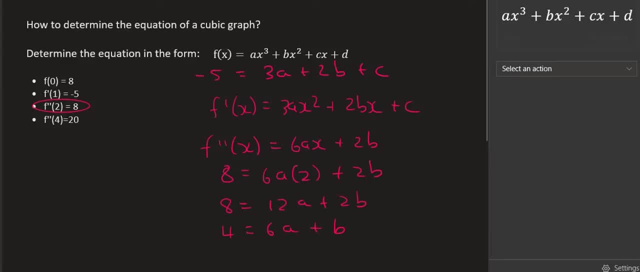 divide everything. But two there just to simplify it nicely. There we go Once again. we can't get any more information, but at least we've plugged it in. So we've got now got two equations that we can use. I'm just going to call them different things so that when I talk about them you 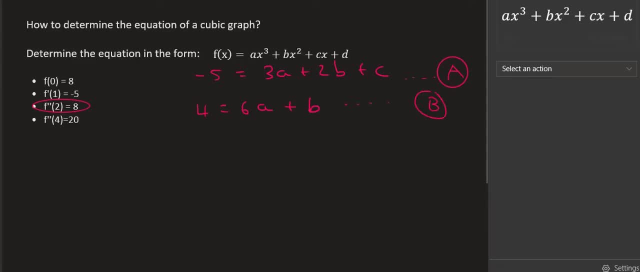 know what I'm talking about. We'll call that one a, we'll call that one b, And then we still have another piece of information to use. So this one we also going to plug into the second derivative on. I've gone and taken it off again, But what it was was six a x. 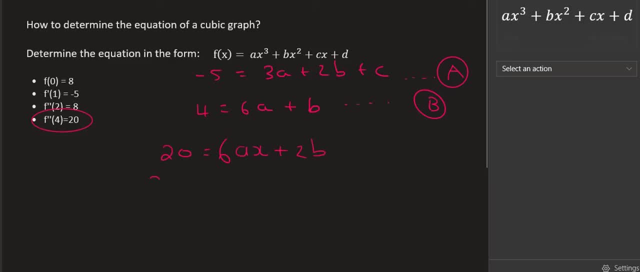 plus two b, And they're telling us that the answer should be 20.. Whenever we plug in an x value of four, So we're going to plug in four, And so that's going to give us 20 equals to 24 a plus two b. I'm. 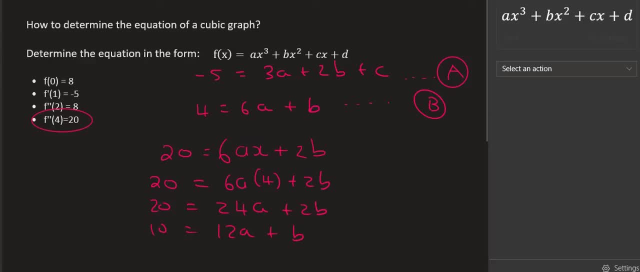 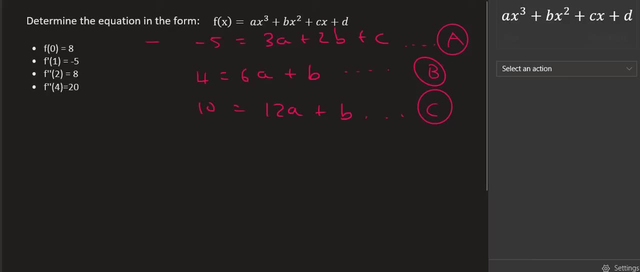 just going to divide everything by two. You don't have to, but it just makes life a bit easier. And there we have another equation. And so there we have it. So have a look at this. We're not going to look at this one over here just yet. Oh, I don't want that to do that. So I've got a triangle. 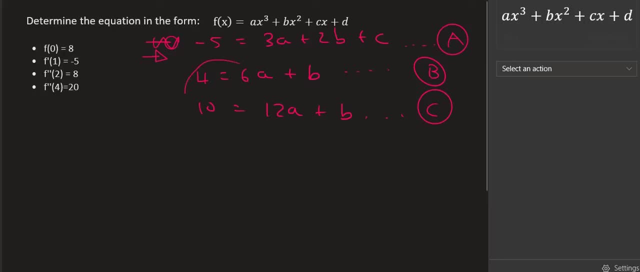 Okay, so we don't want it to, we don't want to look at that one. But if we look at these two, it's two equations and there's two unknowns, a and b, So we just use a simultaneous equation. 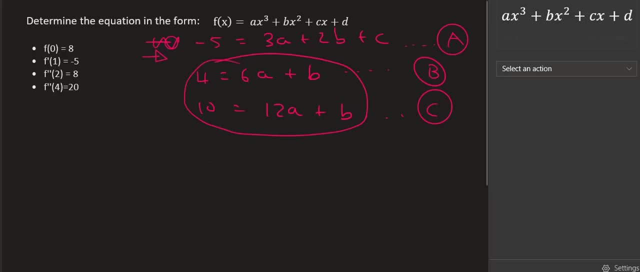 over there. So I'm going to take equation b and I'm just going to rearrange it to become four minus six a. then I'm going to take that expression and plug it in the place of b in the other equation. So it's going to be: 10 equals to 12, a plus. then b is going to be replaced with four minus six a. 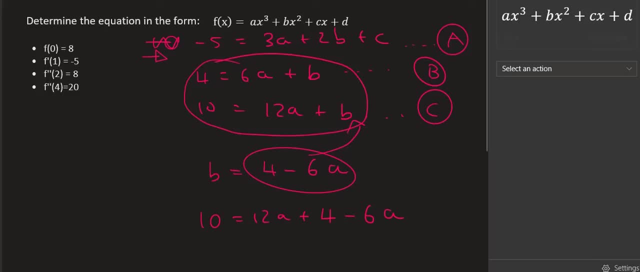 other ways to do this. Many students like to get the b's by themselves. That also works. So then, what we're going to get is six a on the right and six on the left, So a is one I'm then going to. 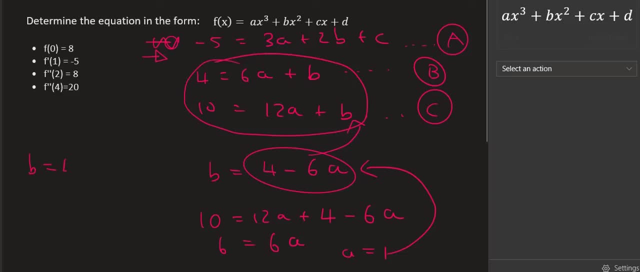 plug that back over there, So that b would be equal to four minus six times one. So b is going to be equal to negative two. Now that we have a and b, we can come back to this equation that was at the top And we just fill in the a value and we fill in the b value, like that, And then 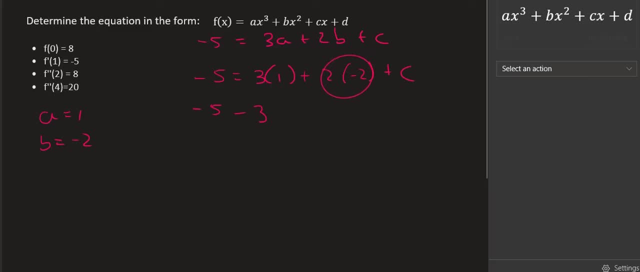 we just bring everything over to the left, That's minus three. This is going to be minus four. So on the left it'll be plus four. So that means c is going to be equal to minus four. Therefore we can say: f of x is going to be equal to one x three. You don't have to say one. 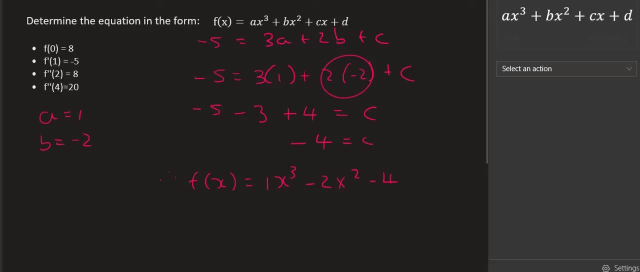 but yes, you can, if you want to. Minus two x squared, minus four x, And we said that d was eight, And there we have our equation. So the most important thing is just go ahead and plug these into the appropriate equation And then we're going to plug in the b value. Equation and then solve.